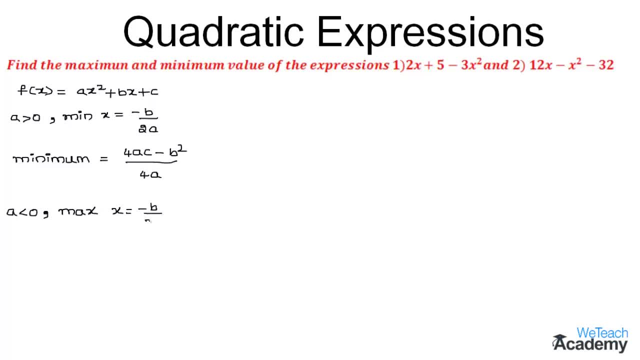 value at x is equal to minus b by 2a And the maximum value of the function f of x would be 4ac minus b, square divided by 4a. Now let us proceed and solve the given expressions. So first let us consider the given expression as f of x. So by writing this expression, 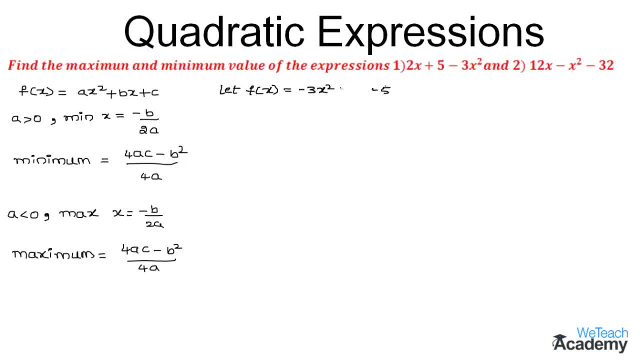 in the standard form, we get minus 3x square plus 2x plus 5.. So, on comparing this expression with a x square plus bx plus c, we get the values of a as minus 3, b as 2 and c as 5.. 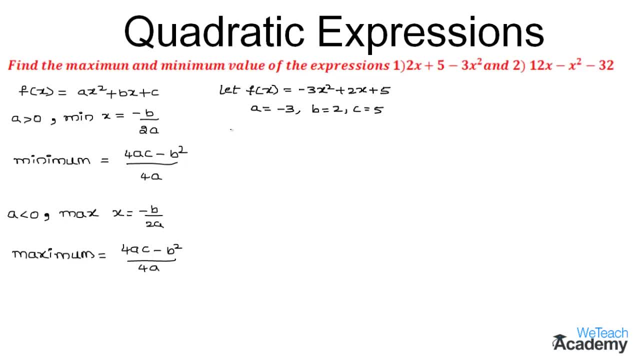 So observe the coefficient of x square, which is minus 3.. So it is less than 0. So we can say that it has. the maximum value at x is equal to minus b by 2a. So here, in this expression, the value of minus b by 2a would be minus 2 divided by. 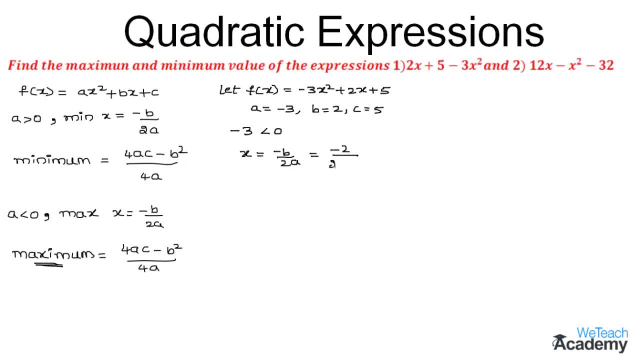 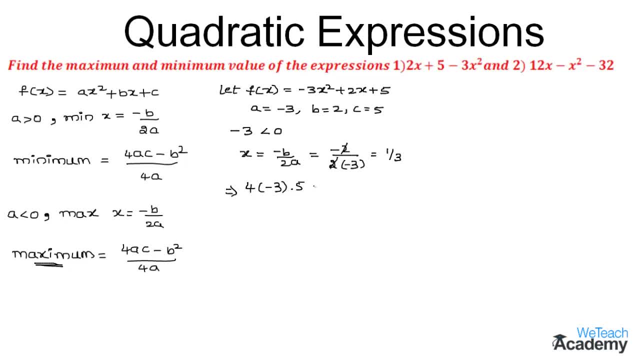 4 into minus 3, into 5 minus 2, whole square divided by 4 into minus 3.. That implies we get here minus 60 minus 4, divided by 4 into minus 3, which would come as minus 12.. So minus 60 minus 4 would come as minus 64 divided by minus 12. and on simplifying this, 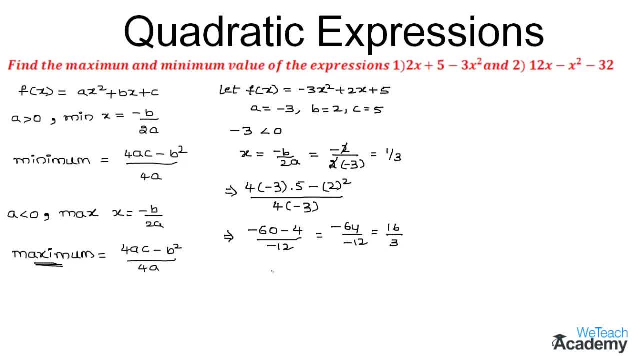 we get its value as 16 divided by 3.. So we can see that the function f of x is maximum at. x is equal to 1 by 3 and the maximum value is 16 divided by 3.. Now let us move over to the next expression.